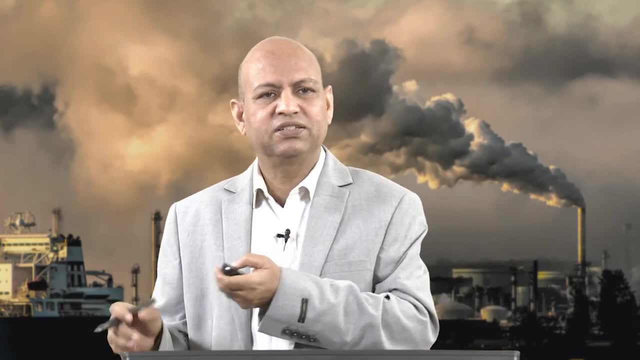 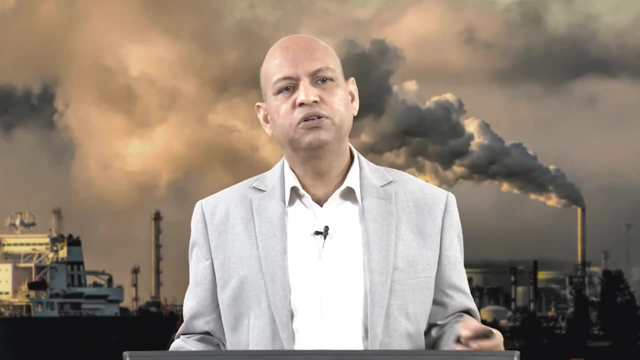 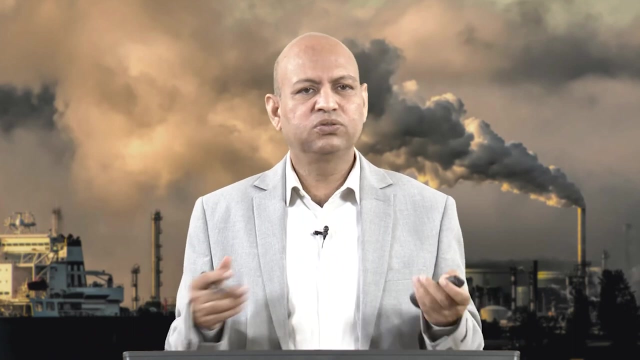 Then pesticides when we are using even for plants, etc. So those kind of exposure may be there From outside also. from outdoor also some pollution can intrude inside the buildings and then some pollution come from surface And those kind of radioactive related pollutants may also be there. 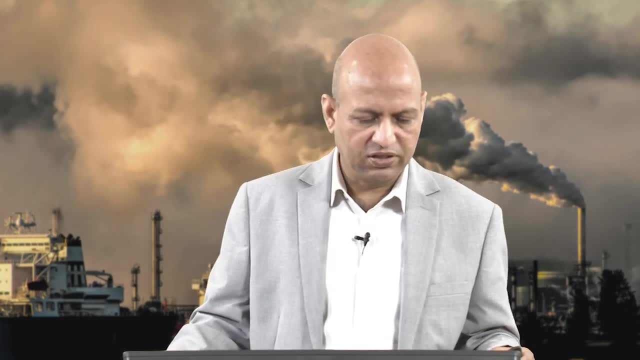 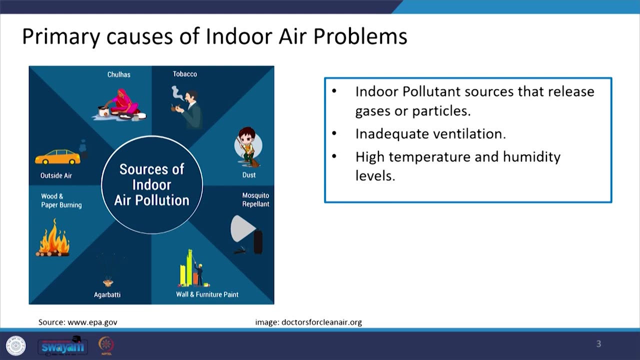 So those kind of specific sources and pollutants we will discuss. So if we focus on primary causes of indoor air problems, then you can see like sources may be many, even from outdoor, like outdoor emissions or outdoor air pollution can also come to the indoor because of like from windows or when we are opening doors, etc. Unless it is very tight building. 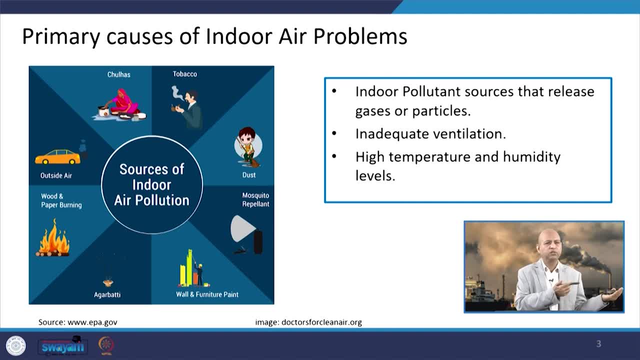 exchange of air can occur, So those kinds of radioactive related pollutants may also be. there is there and, depending upon the outdoor air quality, indoor air quality can be influenced And from indoor emissions outdoor air quality can be influenced, so this is two-way process. 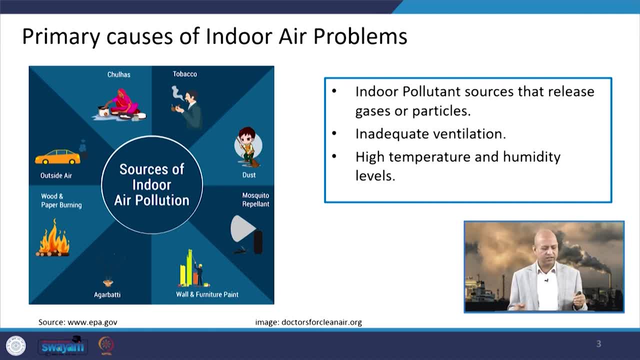 basically, but within the indoor environment, like cooking activity can be there and, depending upon the fuel, whether we are using these biofuels or some solid fuels, cow dunks or wood etc. And if we are using liquid fuels like kerosene or LPG or we are using other kind of stoves. 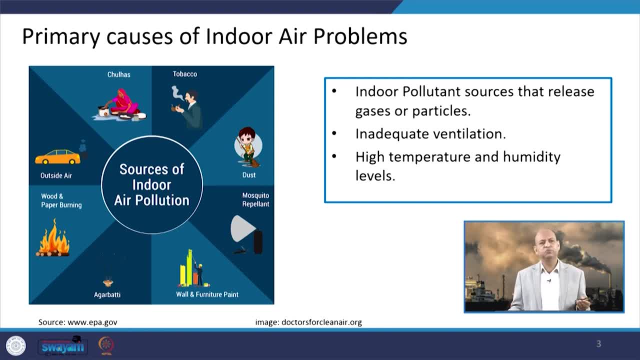 so, depending upon that, some sort of pollutants may come from the kitchen. Well then, tobacco smoking means those people in those families where people smoke, so those contribute to the indoor air quality deterioration because whatever particulate matter or other pollutants are being emitted, they will be inside the house. 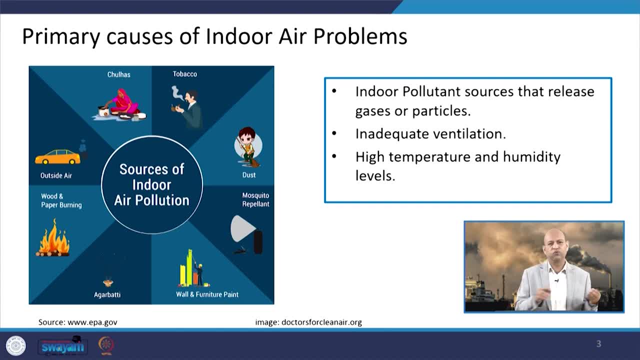 Then you can have this dust, like when you are brooming or you are walking. even then those dust resuspension is there. so that is again another source of indoor air pollution. Mosquito repellents- when we are using some sort of these repellents nowadays, so they 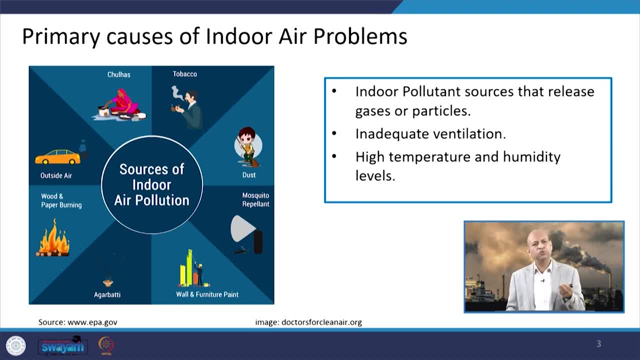 also emit something, some particulate pollutants also and some gaseous pollutants also. When we do some paint related activities, again, some aerosols are there in the air, Yes, The air because of those activities, and even in future also, some paint can emit some sort. 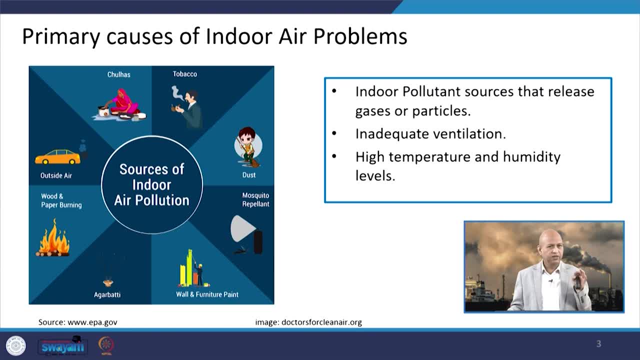 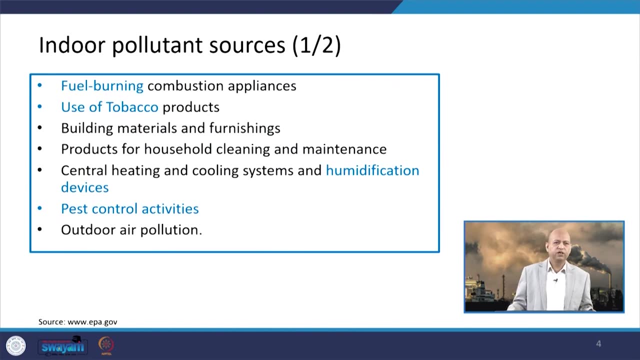 of emissions depending upon what is the composition: chemical composition of the paint, Then, like agarbatti, candle or whatever, the source of the burning is there, so they can contribute to one or other kind of the indoor air pollutants. So the sources are like fuel burning, combustion appliances, use of the tobacco products. 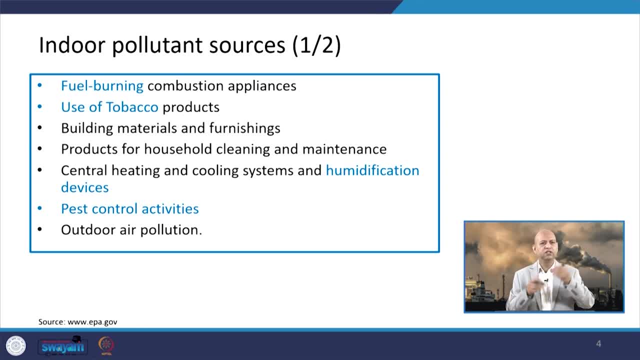 Okay, Then building materials and furnishes- so this is the summary kind of thing which I just discussed- or products for household cleaning and maintenance, central heating and cooling systems and humidification devices. they also contribute. Then pest control activities, because we are using some sort of chemicals. so those chemicals, 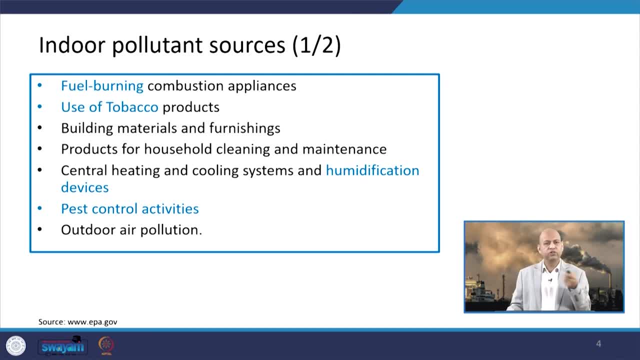 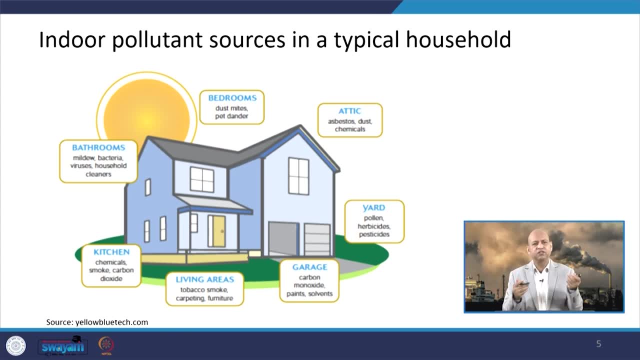 also get emitted into the air and outdoor air pollution. as I said, it can come to the inside. When we try to visualize what things are there, Yes, Yes, Yes, Yes, Yes, Yes, Yes. So we are trying to visualize what is happening inside the building. 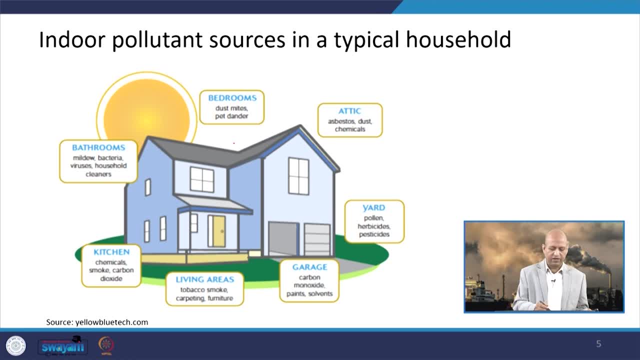 So if this is a kind of residential building, so like dust, mites, etcetera from bedrooms, that can be one source okay. and like pet, then the, because our pet, whether it is cat or dog, they are roaming around inside the building and they can be source of some sort. 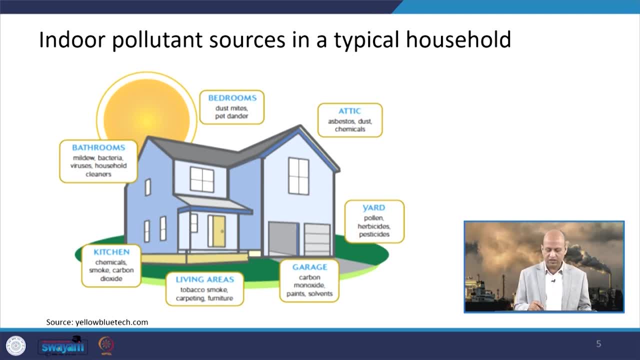 of allergens, etcetera. Then this asbestos and dust chemicals can be from the seats also, then from bathrooms, because several chemicals are being used and moisture is there, humidity is there, so bacteria can also grow, So those kinds of viruses or bacteria can be sourced or emitted from the bathrooms etc. 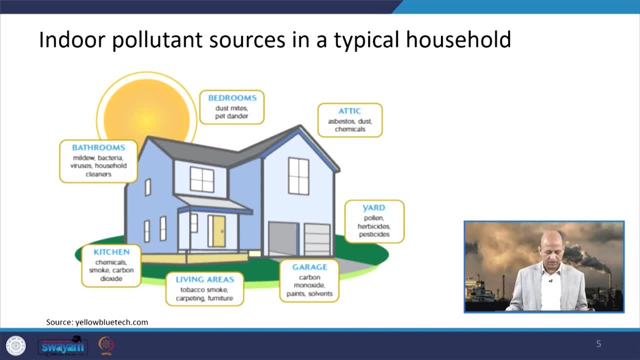 Kitchen can be source of different kinds of smokes, carbon dioxide and other pollutants. Living areas like: if somebody is smoking in the living area then it can be a source of tobacco related pollutants. Garage can be source of like VOCs etc. when some leakage of fuel is there, and yard also. 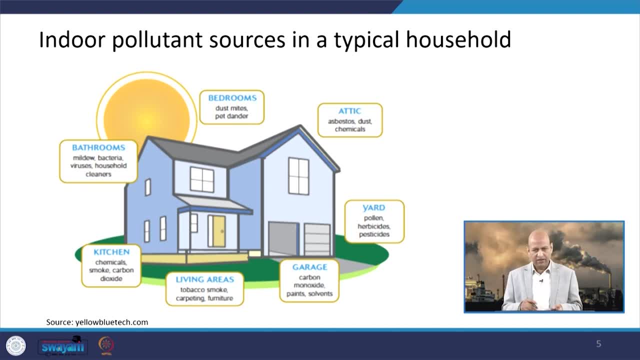 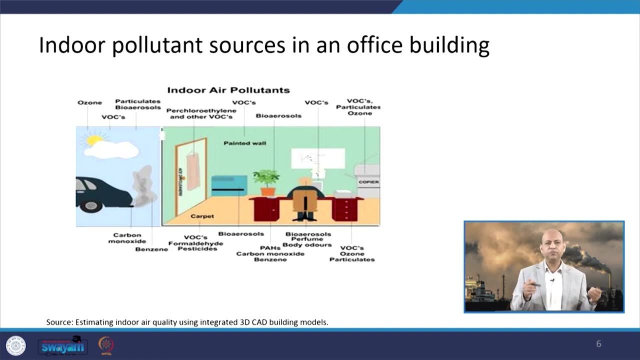 like, because of plants, some pollens may be there, and when we are using some sort of pesticides, so they also come into the air as aerosols. So all these are the kind of sources of indoor air pollution in household related environment When we talk about, like business or office setting. 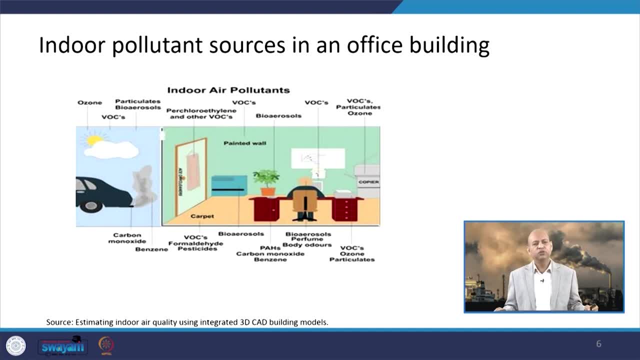 then different kind of activities are there to contribute to indoor air pollution, like photocopying machine is there. So some emissions are there of VOCs. When you are changing that toner again, some aerosols will be in the air and then again similar like mopping and chemicals. we 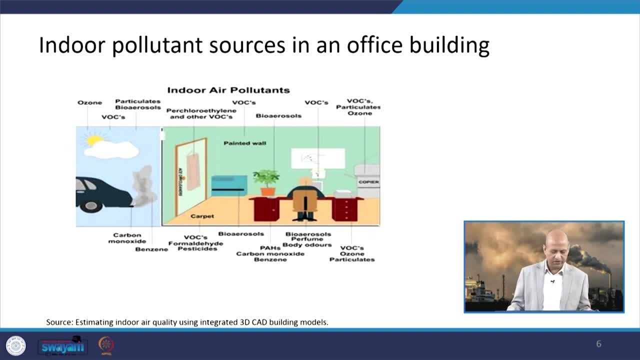 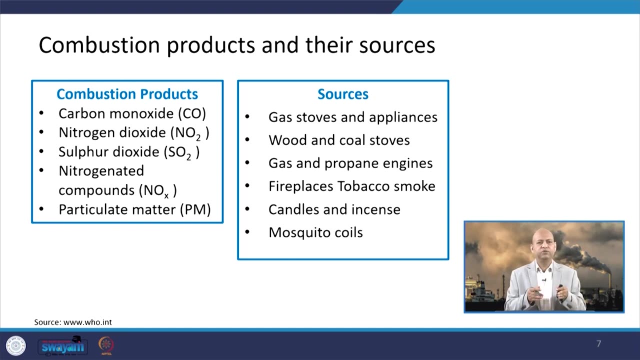 are using, So those VOCs will be in the air and then if it is a laboratory, then other chemicals utilization can contribute to indoor air pollution. Well, so when we relate the combustion products and their sources, this is very comprehensive list, like different kind of. 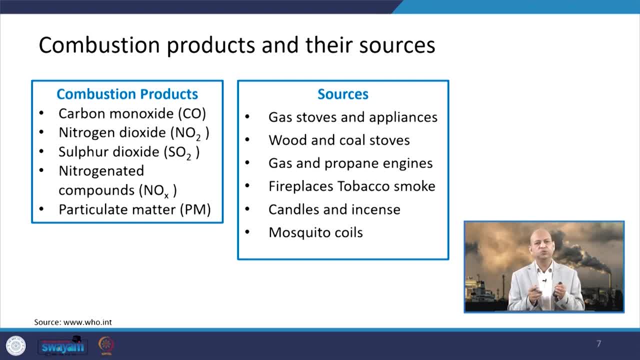 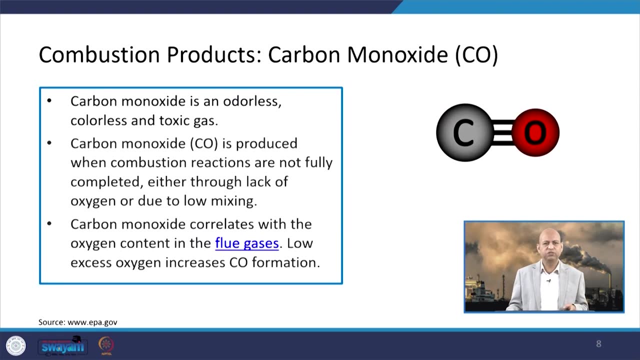 pollutants are there: combustion products, basically like CO, NO2, SO2 and NOx, particulate matter, and they are emitted from gas stoves or appliances, wood and coal stoves or fireplaces or mosquito coils, candles. all those may be the sources inside the house. 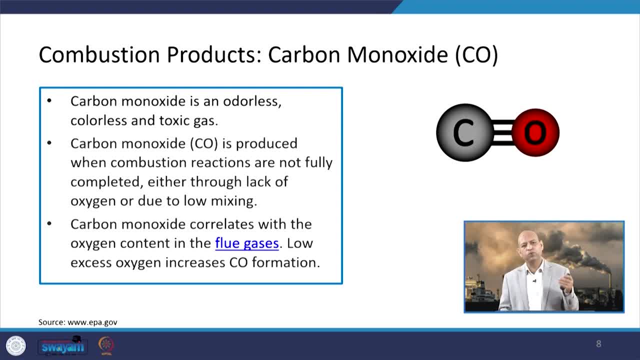 Now if we talk about one by one for different pollutants. So they have certain physicochemical properties, characteristics and the dominating source also for each pollutant we will go in detail now. like carbon monoxide, This is orderless, colourless and but toxic gas. it can go inside our 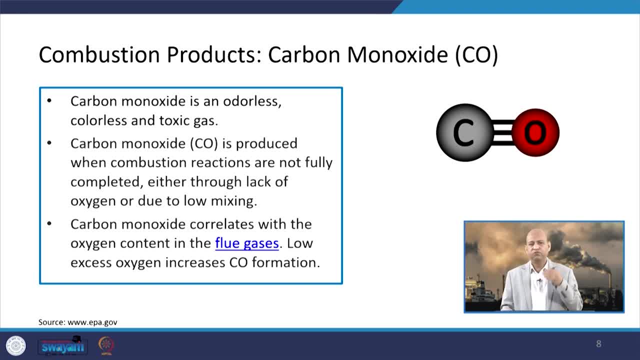 body. it can reduce the oxygen carrying capacity of the blood. we can get unconscious. even high dose can kill the persons, is a silent killer because it does not smell and it is difficult to detect. it poisons and it can kill. Well then, there may be certain sources for that. for example, you can see here all these: 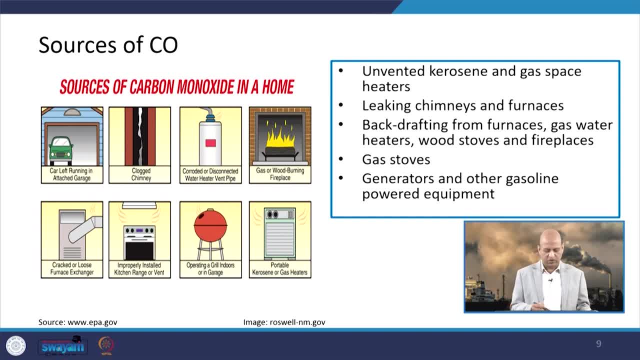 kind of sources are there which contribute to the carbon monoxide emissions, whether it is gas or wood burning fireplace or car left running in the attached garage, so carbon monoxide is there in the these exhaust emissions. All these activities can contribute to the CO emissions. 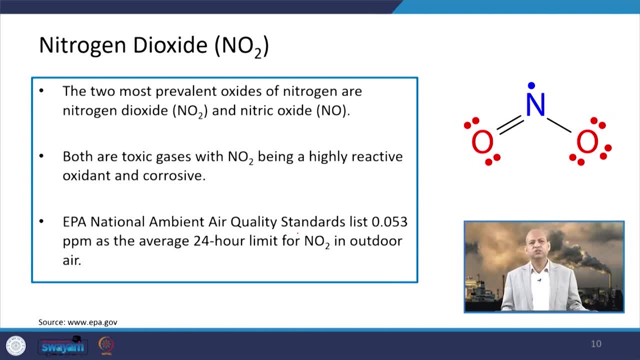 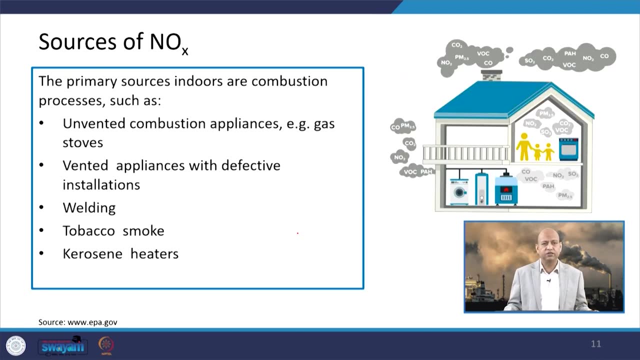 When we talk about nitrogen dioxide. so this is the. whether it is NO2 or NO, these are having negative health effects and this EPA, National Ambient Air Quality. they have given certain standards and beyond that they are quite toxic, basically reactive. and the sources: 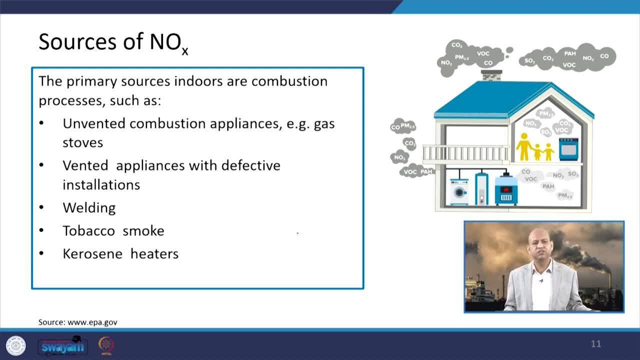 could be many again as, like unventilated combustion appliances, gas stoves, etcetera, they emit loads. So there is a lot of NOx, because NOx emission is always there, like CO and CO2 is there whenever you are burning something, because NOx has to be there when burning activity is nothing. 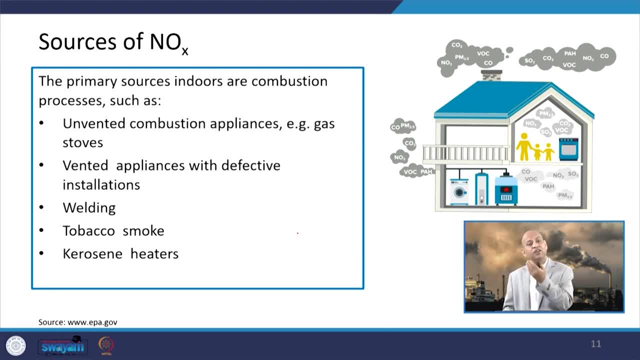 but oxidation and oxygen is coming from the air and in air lot of nitrogen is there. So NOx emissions excluding is very, very difficult, unless you capture that and convert into something else through catalytic converters, etcetera. otherwise NOx emissions are there. 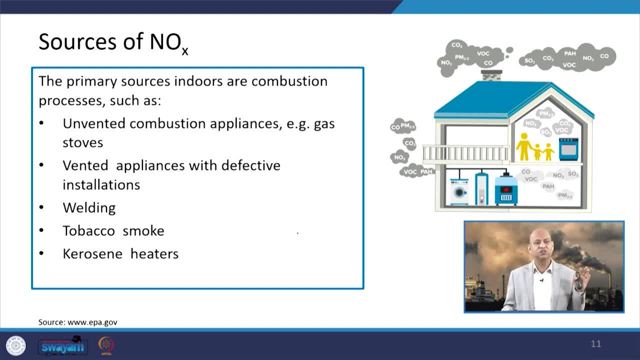 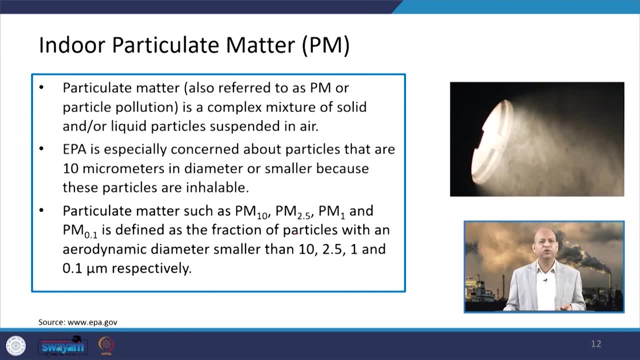 You can control many emissions, but NOx emissions control very little. Controlling is a very difficult task. basically, well, from welding, tobacco smoke, kerosene, heaters, all these are sources for the NOx emissions When we talk about the particulate matter. so they also come from different sources and 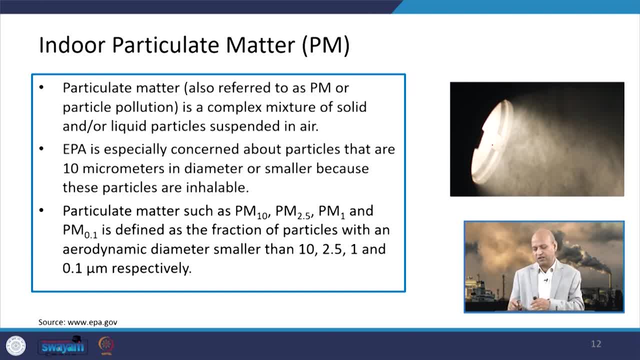 you can see, like when sunlight is coming in a dark place. you can see different small particles which are detectable by naked eye, but they may be very small particles, ultra fine particles which are not visible, very, very fine particles. We can talk about nanoparticles also, and they can go into our body, into our blood. 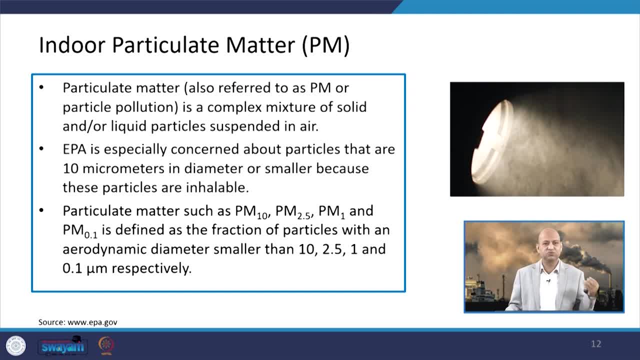 also, And if they are toxic they can really trigger some very chronic diseases, And there are certain standards and we have to be careful that the concentration, whether indoor or outdoor pollution of these particulate matter, etcetera, etcetera, should not exceed. 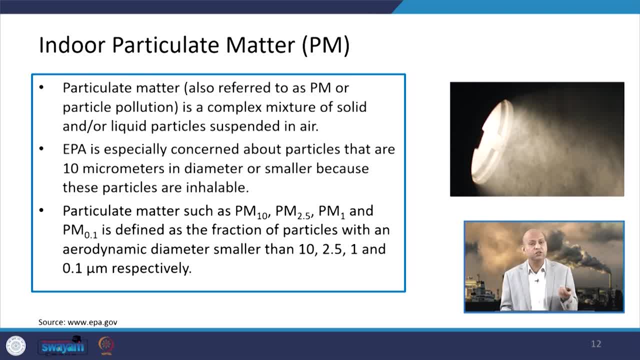 beyond that standards, but it may exceed, depending upon the strength of the source. And then So the size and shape of the pollutants of the particulate nature also govern the health impacts, like PM10, PM2.5, PM1, they have different range of affecting our health because they 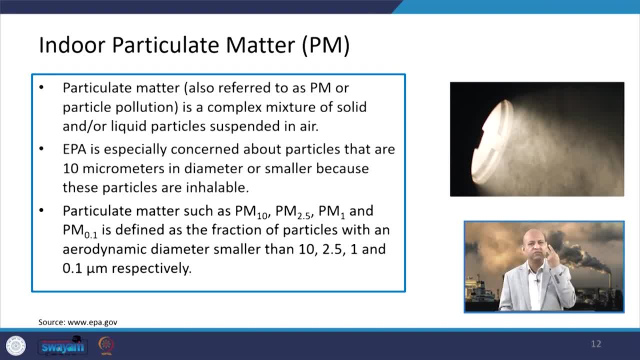 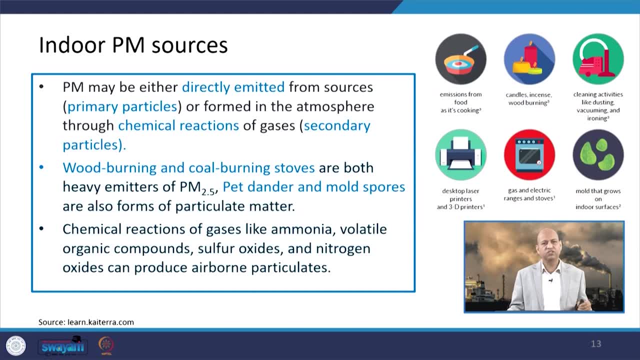 are respirable. Coarser may be removed by our nostril, this filter system, but small particles can go to respiratory system and influence our health. as we discuss normally about these, Then indoor PM sources are many. Whatever burning activity or We are walking, even then some suspension is there. 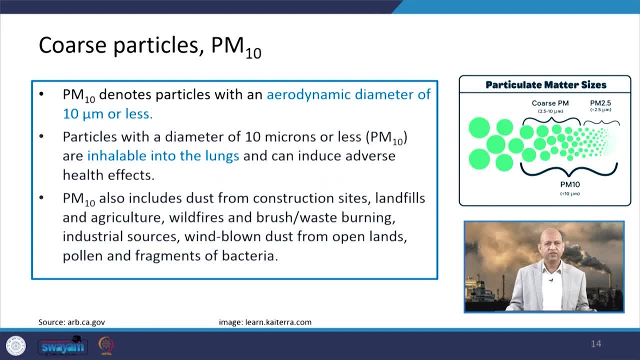 So all those sources are there for particulate matter And the coarse particles and the PM10,. they have different nature, as I said, and they have different health effects. So we need to be careful about small or fine particles, basically like PM2.5 and you can. 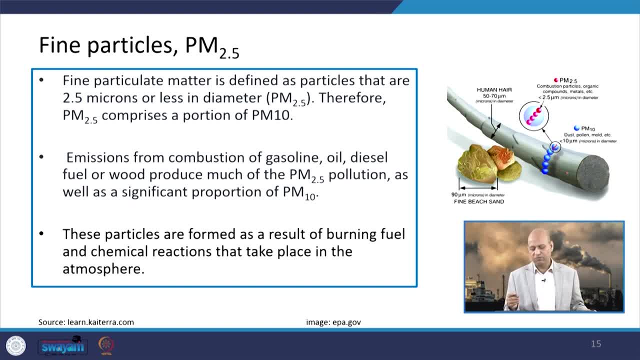 see the comparison with this human hair. what is the size of these fine particles? So you can appreciate these are very, very smaller or very fine particles which are very, very small. These are the particles which are difficult to imagine or look at and visualize. 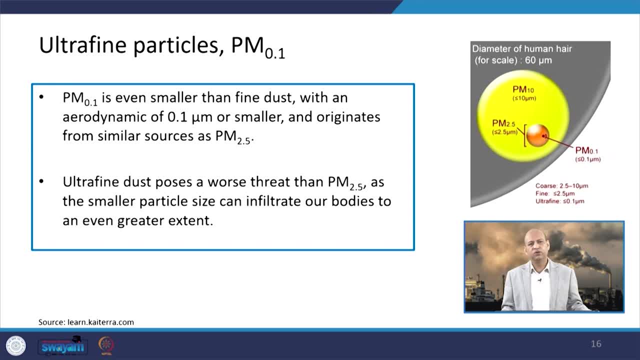 Well, ultra-fine particles like 0.1, PM0.1, they are very smaller and they can originate from similar sources like PM2.5, and they can pose very threatening like more than PM2.5.. And as it is very small particles and can infiltrate in our bodies. 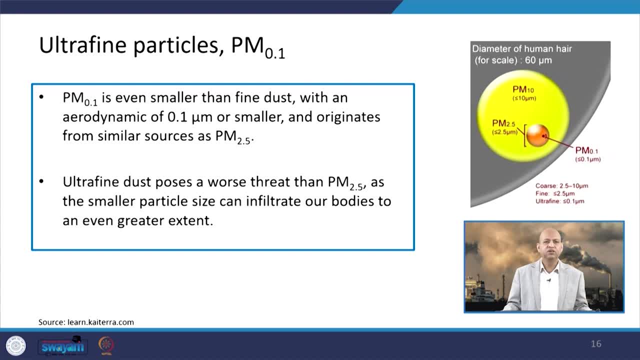 So we need to be careful about these, So we need to be careful about these, So we need to be careful about these So we can paradise these to the greater extent. So we have to be careful about the presence of these kind of very small particles and 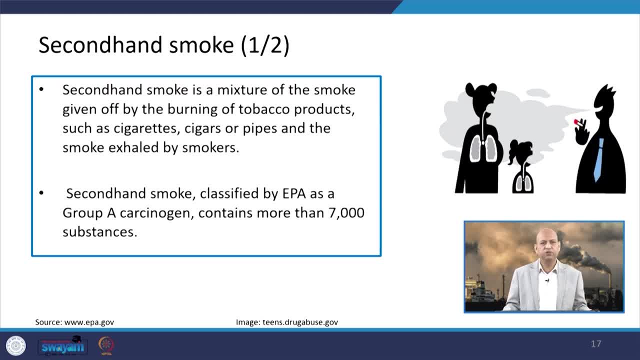 if they are present, then we should do something to remove them from our indoor environment. When we talk about this secondhand smoke which is coming from like smoking activities, So the passive smoking is there because, even if you are non-smoker, somebody smoking and 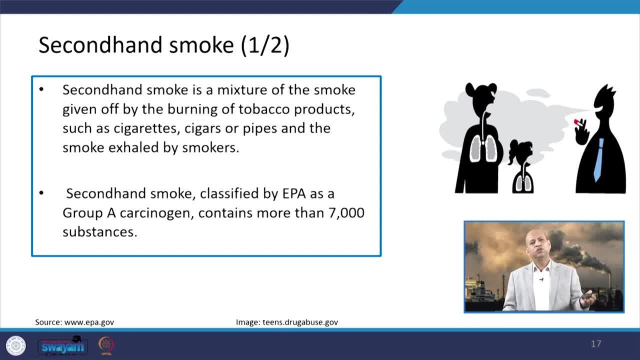 in the air, those particles, those gaseous components are there, you are inhaling and that way again you are exposed to the chemicals, exposed to those pollutants which are dangerous to your health. So this kind of secondhand smoke sources can also be there and you can see like middle 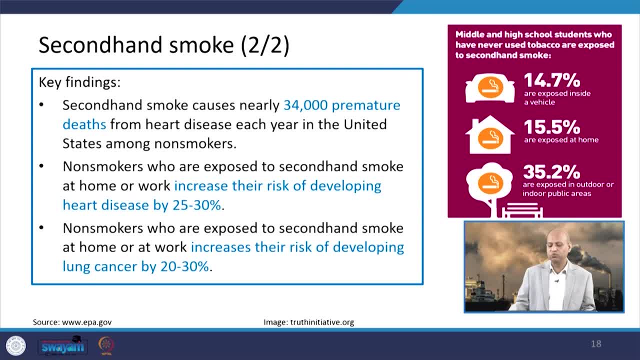 and high school students who have never used tobacco are exposed to secondhand smoke, that is, the passive smoking. Around 15 percent are exposed inside a vehicle- some adults may smoke, may be smoking there, So this is not good thing- And around 16 percent are exposed at the home. 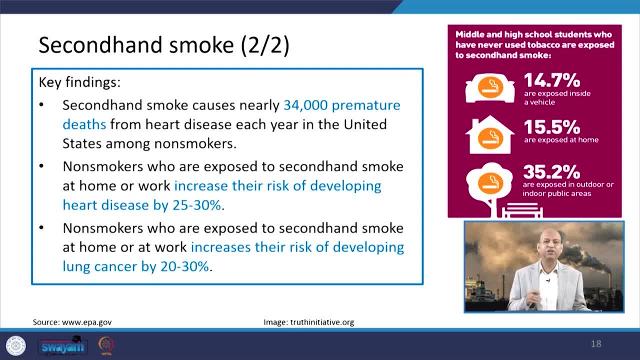 And more than 35 percent are exposed in outdoor or indoor public areas where people are smoking. So that way also nowadays, lot of regulations are coming and specific places are there for smoking and public places are prohibited from smoking, but still some there are ways because 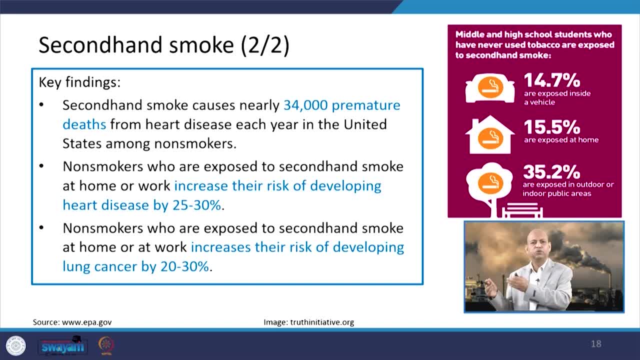 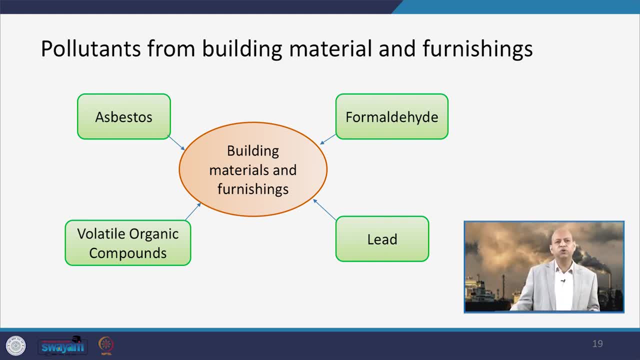 it is difficult to control the air pollutants. They can travel depending upon, Depending upon the wind direction and wind velocity. So in totality, if we talk about like pollutants from building material and furnishing, then different kind of pollutants may be there, like asbestos, formaldehyde, volatile organic 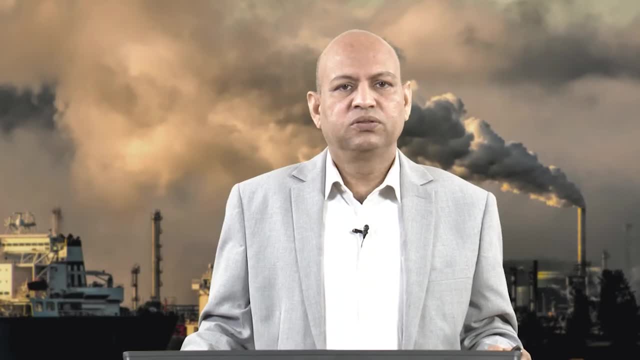 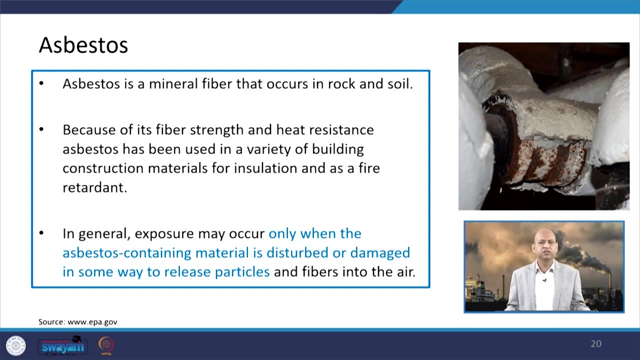 compounds or lead, those kind of things. So these are the different pollutants and, if we go one by one again, so the asbestos is basically. these are coming from mineral fibers and that occurs in rocks and soil, but they may be like from seeds, wherever they are present, so they can get emitted. 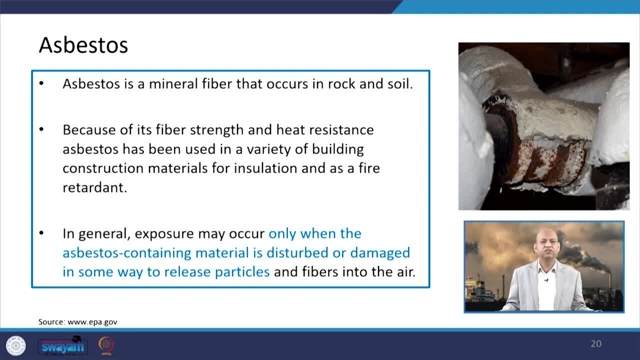 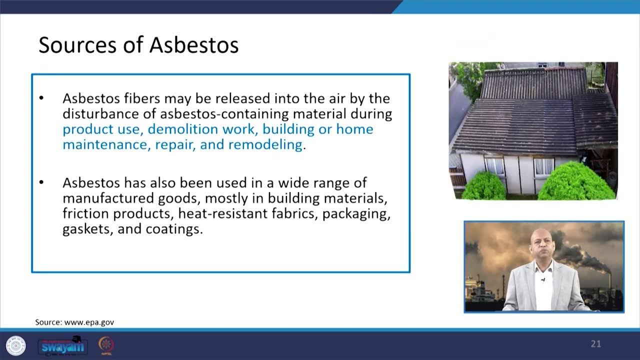 in the air And exposure may occur when these asbestos containing material is disturbed or damaged in some way. then the particles are released and they becomes in the air and they can be part of our respiratory. this inhalation Sources of asbestos can be different seeds, whatever building material which they are. 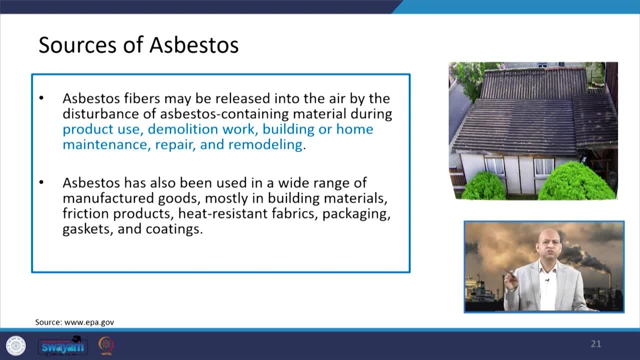 using the asbestos. So those kind of things, Okay, So those kind of tiles or sheets- they may be there for these releasing asbestos, These heat resistant fabrics or packaging, gaskets, coatings, all these, they are using the asbestos. 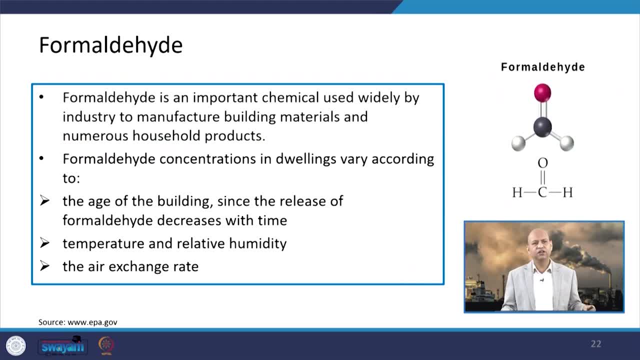 So means it is present there, basically, so it can get released from there. Formaldehyde can be there like it is a very important chemical and it is widely used in industry to manufacture building materials. So again, it will come from the building material basically. 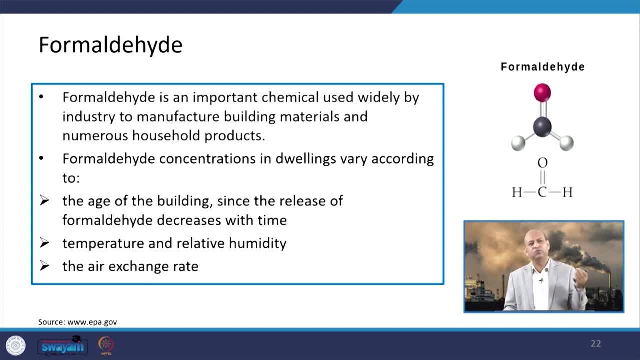 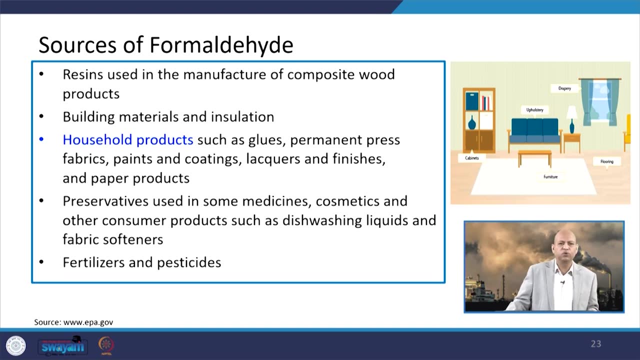 And like different concentrations in dwelling units depending upon the age of the building, and the release of the formaldehyde can decrease with the time. The temperature, relative humidity, all these influence the concentration into the air And the sources can be all those kind of household products like glues, permanent pressed fabrics. 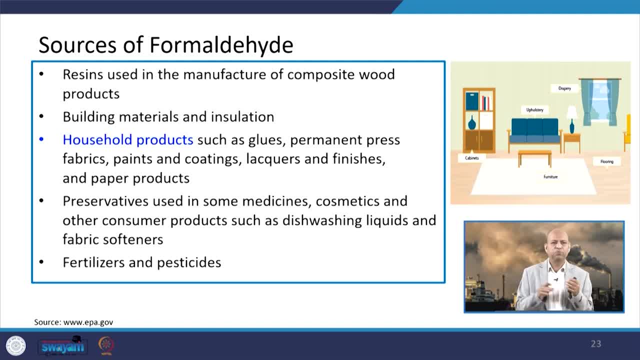 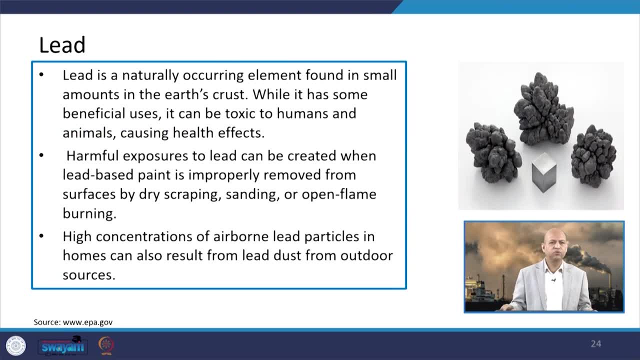 paints, coatings, all these finishes, paper products. they are using all those kind of things where this formaldehyde may be present, Okay, And they can come out depending upon the temperature, etc. Similarly, lead is present in different kind of things like paints, etc. 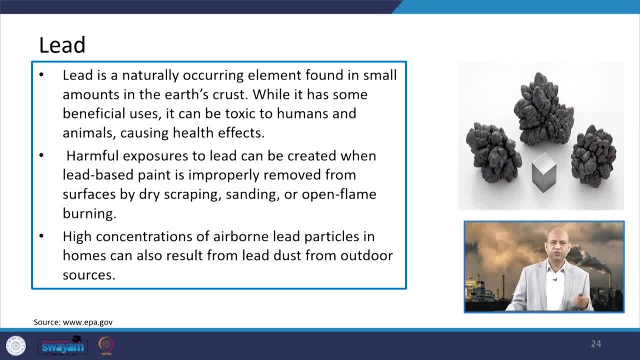 That is why this, nowadays, unleaded paint, is becoming popular, Like unleaded petrol or unleaded gasoline. it used to have a lot of lead content, but there this new policy came into existence because lead is very harmful for this memory growth or brain growth in the body. 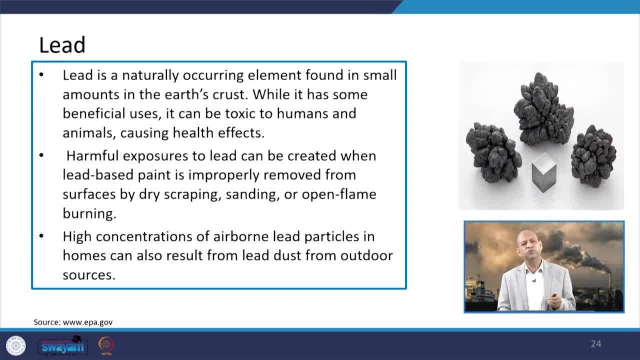 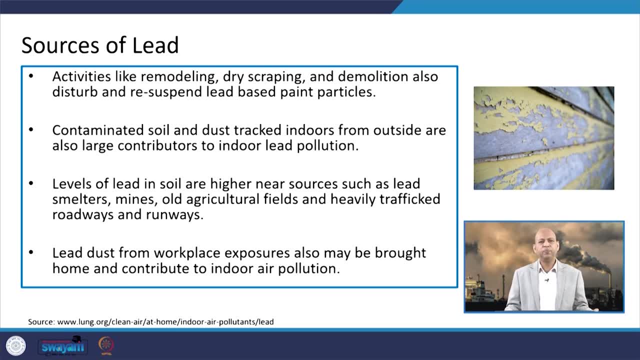 Okay, Children. So it was reduced and it is now very, very negligible kind of thing. Right, Then sources of the lead can be like you can see: scraping, demolition, disturbance of those paint related things- then the lead can get emitted into the air. 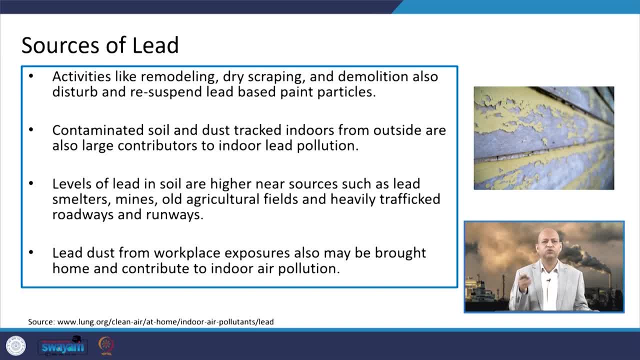 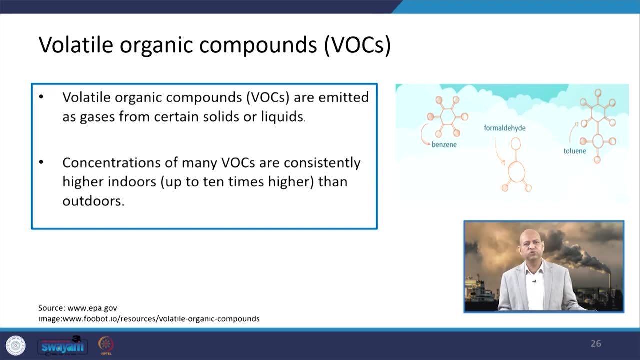 Okay, And it can be also through smelters or mines, old agricultural fields. so there, if it comes to the outdoor And if some from outdoor air also it can go inside the buildings in workplaces. When we talk about volatile organic compounds, VOCs, so they can also come from paints etc. 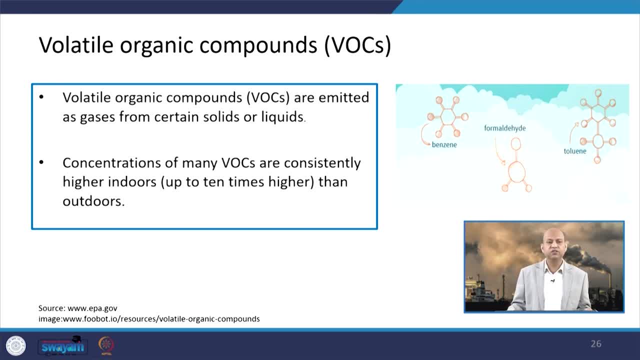 Right. So, like in indoor environment, it is 10 times more than the outdoors. So this is very dangerous because many people are allergic to VOCs, Okay, And this is not good for health, So we should be careful about their concentration. 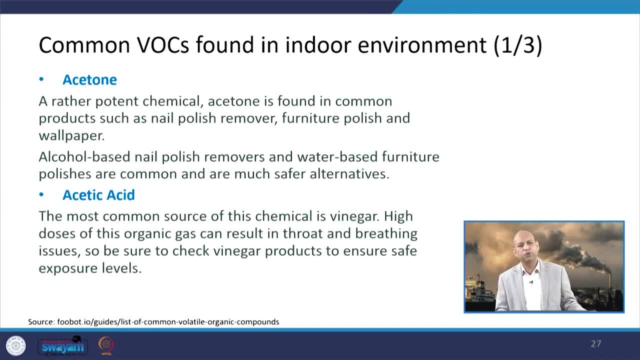 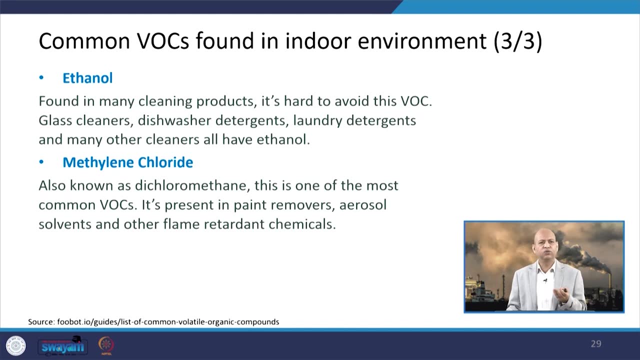 They should not go beyond the environment. Okay, They should not go beyond allowed or permissible levels. When we talk about like categories of VOCs, there are many like acetone, acetic acid, all those kind of like butanil or carbon disulfide, and then ethanol or methylene chloride. 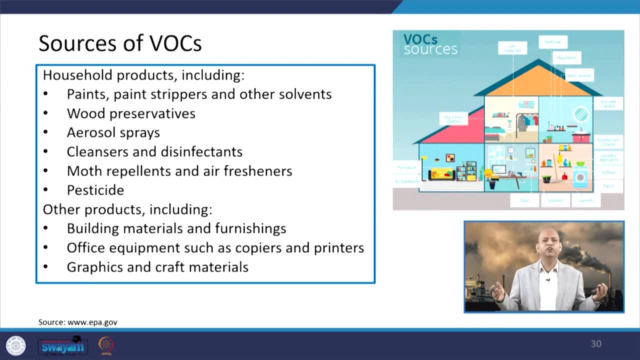 Okay, All these are there which are having different kind of health impacts on the body, And household products which include these VOCs are like paints or wood preservatives. Okay, Aerosol sprays. So whenever you are going to have like good spray which smells good in the indoor environment, 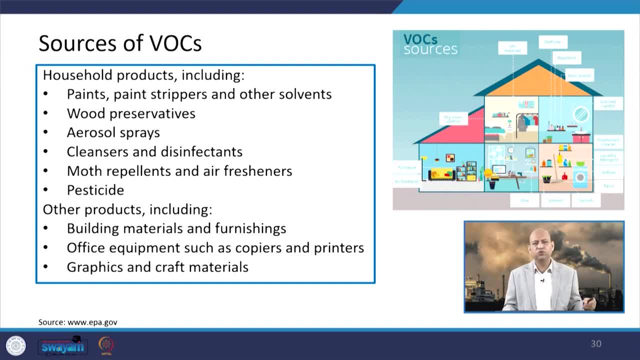 but it is not good for the health because it is having these toxic VOCs. Okay, And then these cleanliness and disinfectants- they also have these kind of VOCs. Moth replants or air fresheners, as I said, pesticides- all those can be source of VOCs. 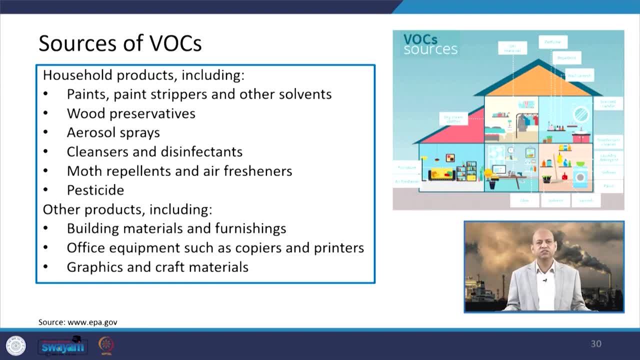 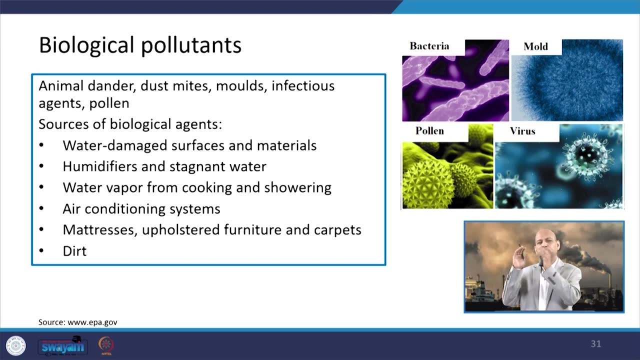 Okay, Other products of like building materials and furnitures, office equipment such as copiers, photocopiers, printers, graphics and craft materials- all these can be the source of VOCs. Well now, if you talk about biological pollutants, which can come from humid corners or moisture, 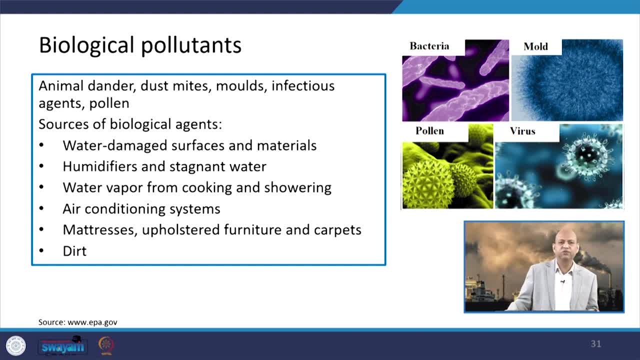 or leakage, seepage, etc. that kind of thing is available or present in the building. that is not a healthy sign of the building, Right? Okay, So these surfaces, materials, humidifiers, stagnant water- they can be source of biological. 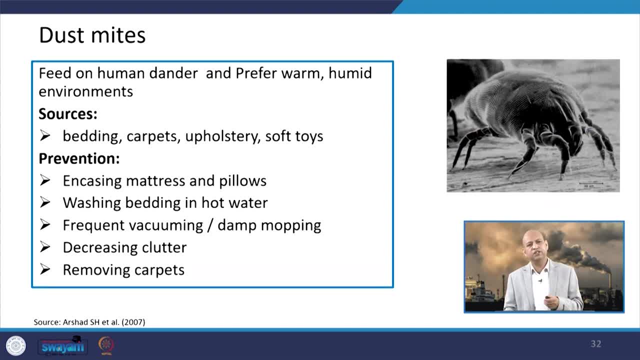 pollutants, basically, And like dust mites, may be there. if we are not cleaning bed sheets and the bed periodically, if you do not vacuum it properly, then these kinds of dust mites may be there and they are very allergic and they have those kinds of effects. 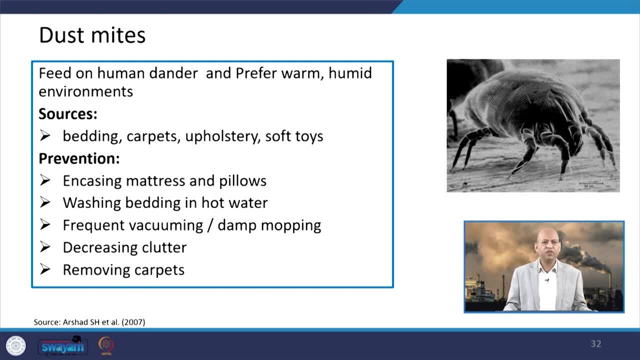 Well then, if you want to prevent them, then you should go for better mattresses, Okay, And pillows, washing them regularly, cleaning them properly, and we should not have much clutter in the room where we are using it for longer periods, and we should not have. 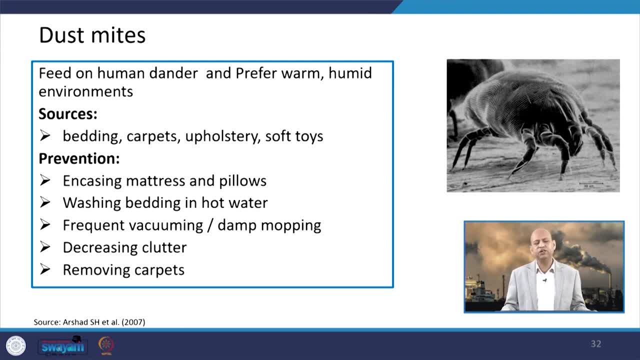 the carpets. basically, if we cannot maintain it, Carpets can be a big source of small particles or these biological pollutants or dust mites etc. if you do not vacuum it very regularly. So instead of carpets it is better to have the tiles. 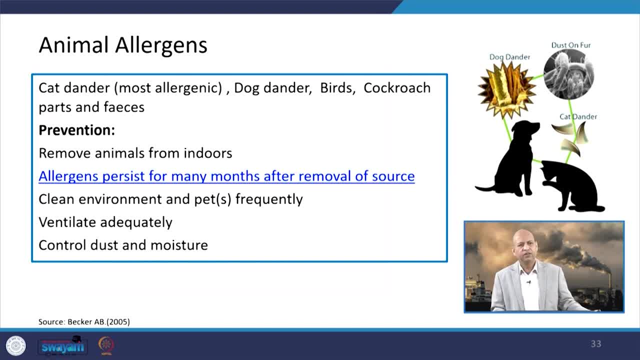 You can clean it regularly very easily, comfortably. When we talk about like animal allergens, so from like cats or dogs, from waste or their hair fall, all those can contribute, even cockroach, etc. birds- many people have birds. 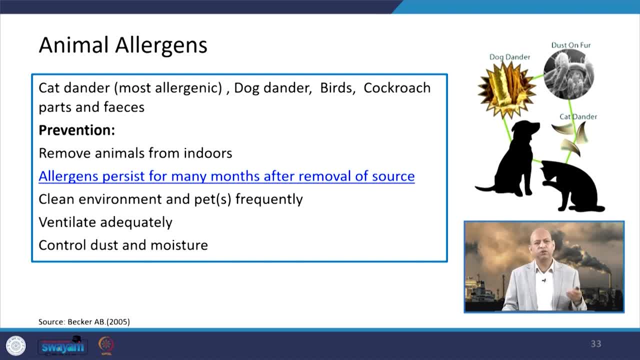 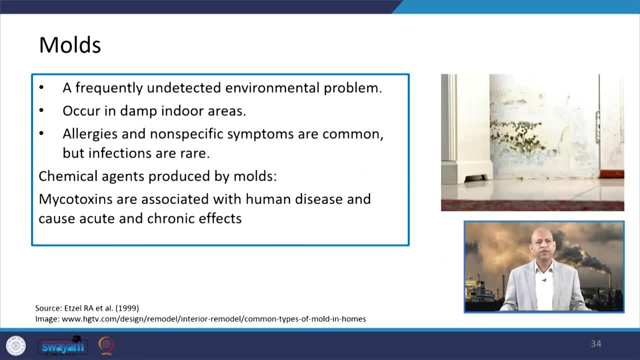 also. So those are. if they are in the indoor environment, they can contribute these kinds of allergens which come from their hair, fall, etc. Then moulds can be there, As I said. So these moist corners or these leakages or seepage related corners, so various kinds. 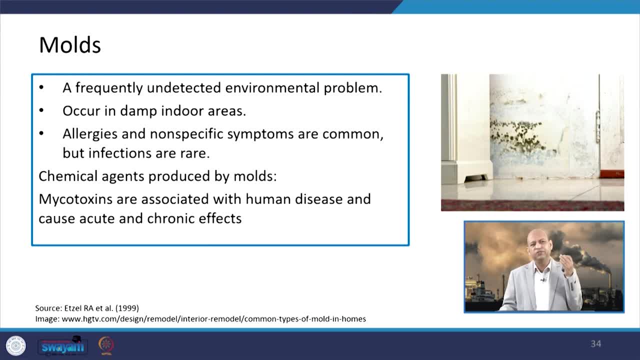 of moulds have different kind of allergies to people. Many people, if they enter- and this moulds kind of thing is there- they start sneezing, Their eyes get red and those kind of symptoms may occur because of these VOCs as well as. 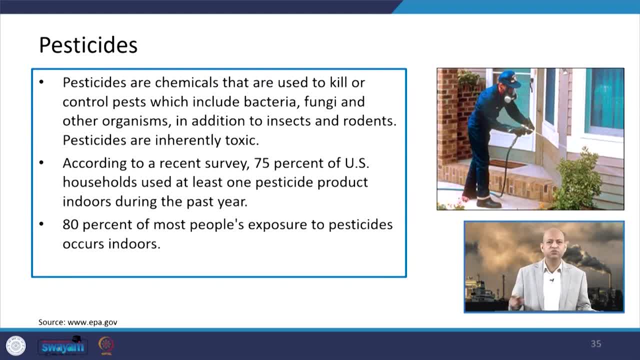 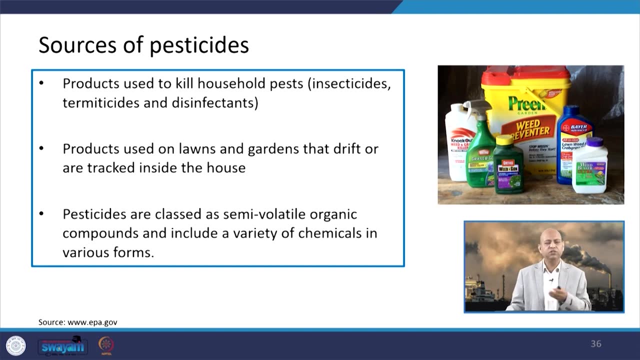 these moulds kind of thing, Then pesticides may be there when you are using for gardening etc. So that can also go inside the building, because we have indoor plants also and sometimes we use pesticides etc. So the sources of the pesticides can be all these kind of chemicals which we are using. 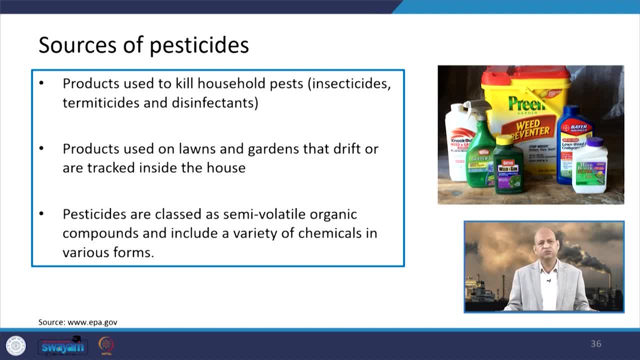 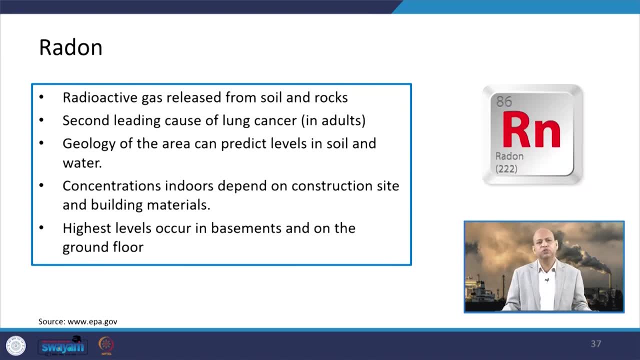 to protect the plants and to repel those unwanted kind of pest, etc. Well, radon, radioactive gas, can be released from the soil and rocks and this is the second leading cause of the lung cancer in adults. So this is the second leading cause of lung cancer. 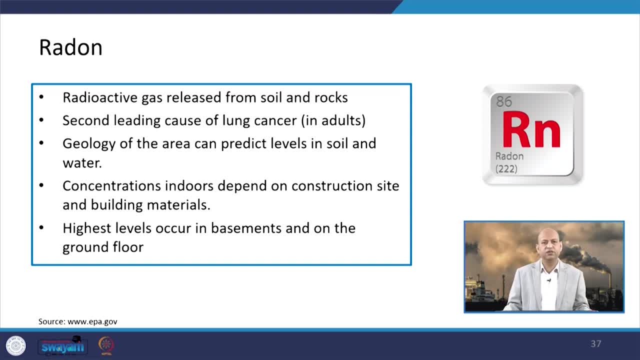 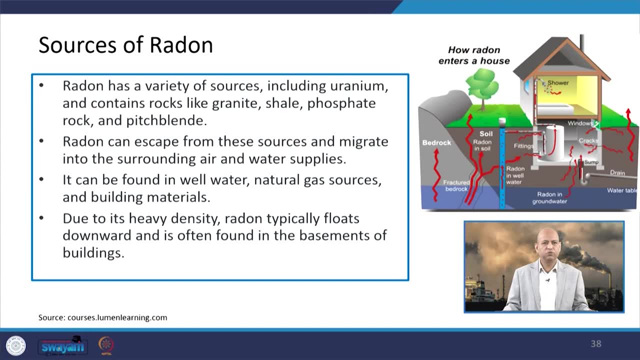 So the geological formations of that particular area can influence this radon presence in particular localities. So if it is present then one should take care, otherwise it can influence the health and later on even cancer related problems may also occur. So the sources can be different: rocks or these kind of granite or shale or phosphate. 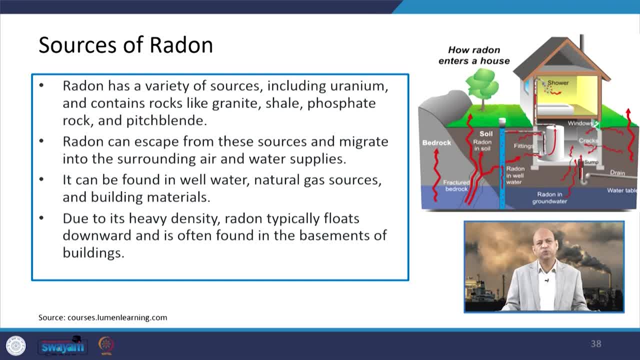 all those kind of rocks can have These particular pollutants or radioactive entities. Well, so, due to the heavy density of the, this radon, they typically floats downward. It is often found in the basement buildings. So if somebody is spending a lot of time in the basement and if you find that radon, 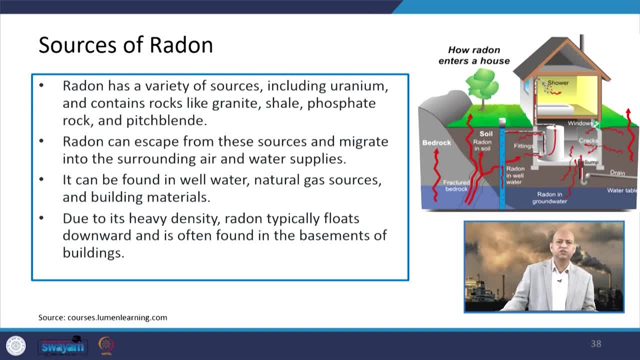 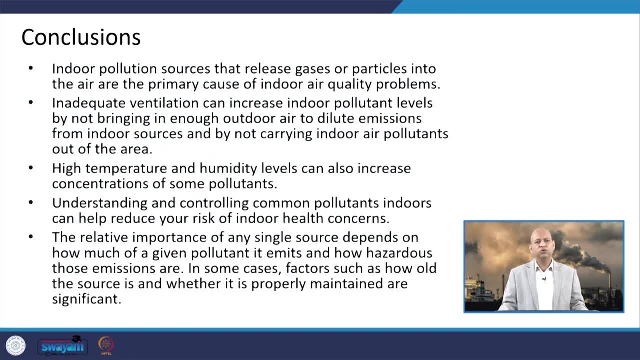 is present, then it is better that you make it fully ventilated and flush it out, otherwise it may be very problematic. So this is the second leading cause. So all in all, we can say that indoor air pollution is a big problem and there are specific 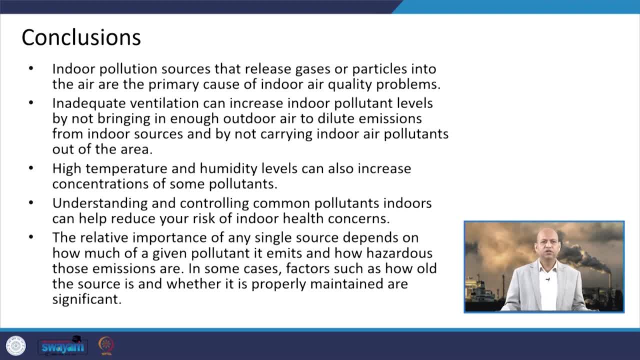 sources for some specific air pollutants which are significant in indoor environment and it can vary from household to the office kind of setting And accordingly we have to be careful about their monitoring and their levels and they should not go beyond those kind of levels which can be health hazard. 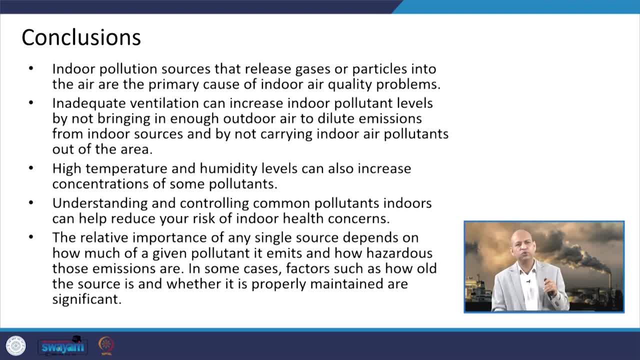 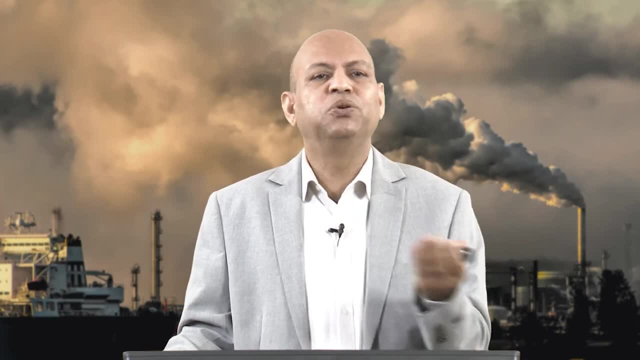 So the knowledge about these specific sources- Okay, So the knowledge about these specific sources and specific pollutants, of indoor air pollutants, can give us an idea how to keep our environment, micro environment, indoor environments- clean and we remain healthy, because nowadays lifestyle is such that the most people live indoors.